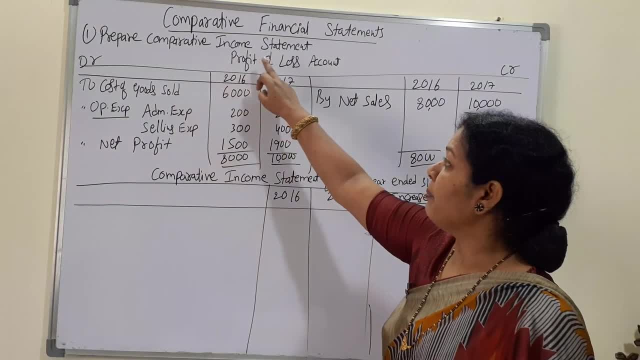 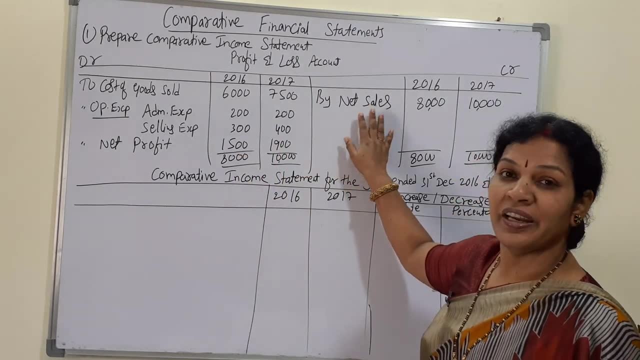 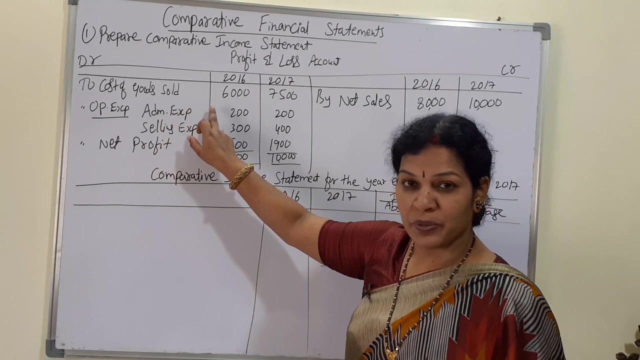 let's see the problem and problem I have taken: prepare, compare, prepare comparative income statement. what is given profit and loss account. in profit and loss account, credit side- net sales two years 2016 and 17 and debit side cost of goods sold, operating expenses, administrative expenses and selling. 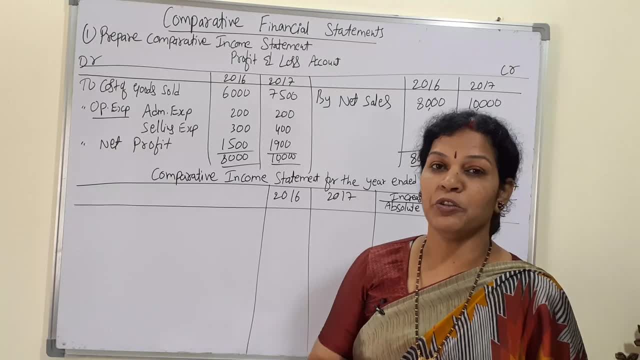 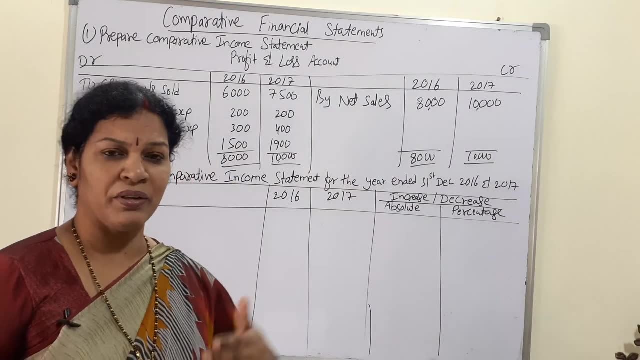 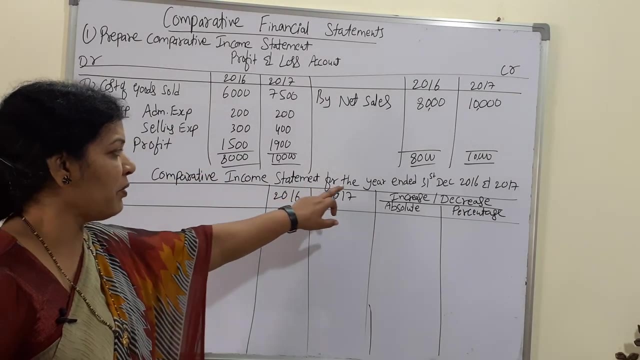 expenses and net profit is given to us. so what we need to prepare is comparative income statement for this. the performer is same, like schedule of changes in working capital. already we have done in funds flow statement: same kind of performer. this is so what I have written here: comparative income statement for the year ended 31st. 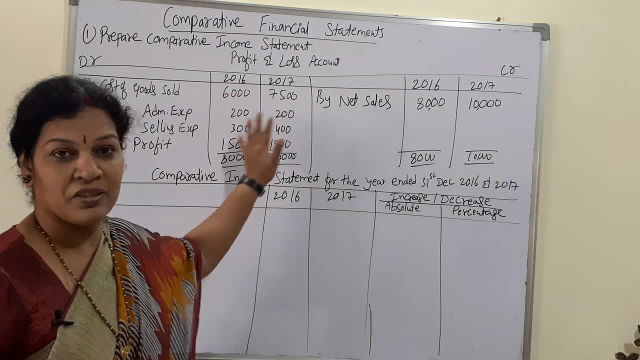 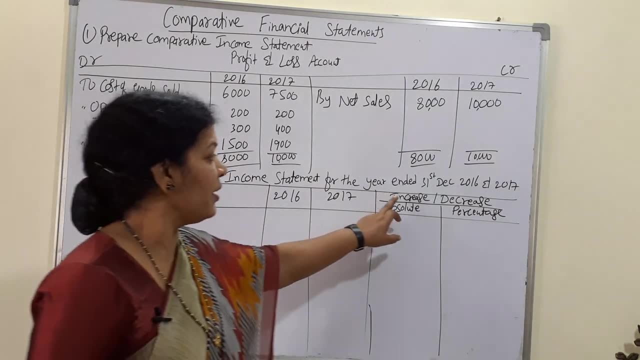 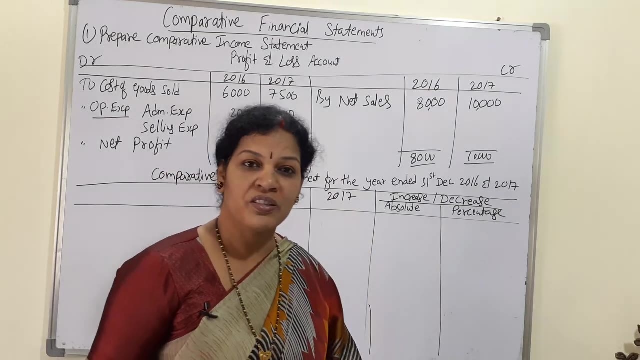 December 2016 and 2017, both the years comparative statement I'm preparing. so here particulars will write 2016-17, and here increase or decrease, absolute means how much is increased and percentage wise will write. so first, to prepare this comparative income statement will take first. 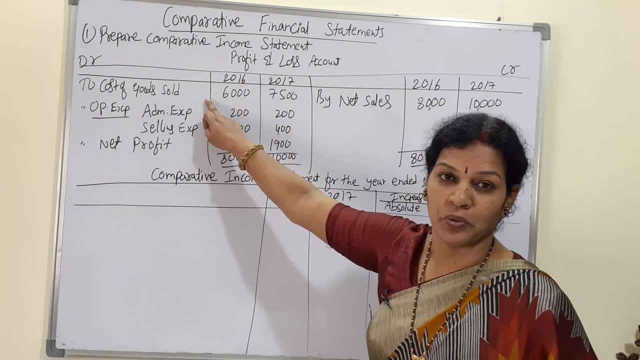 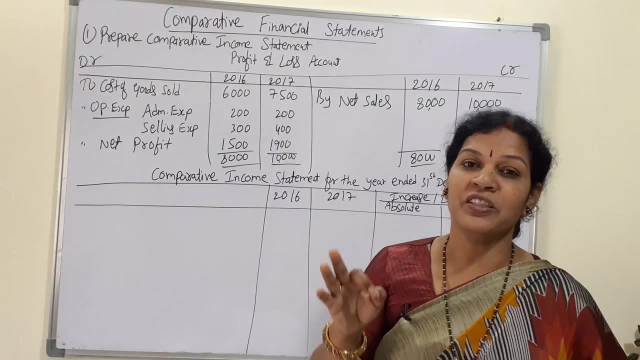 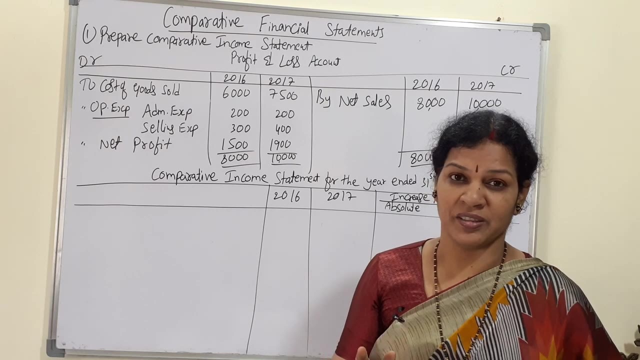 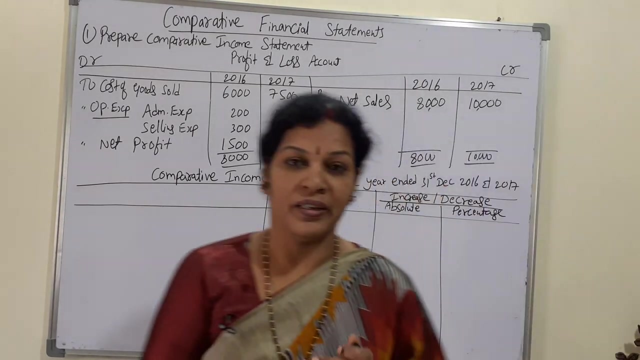 net sales. net sales minus cost of goods sold. net sales minus cost of goods sold will be getting gross profit. once if we get the gross profit will deduct the expenses which are related to the indirect, indirect expenses. then will come to know net profit or operating profit. we can say so first what we'll do: net 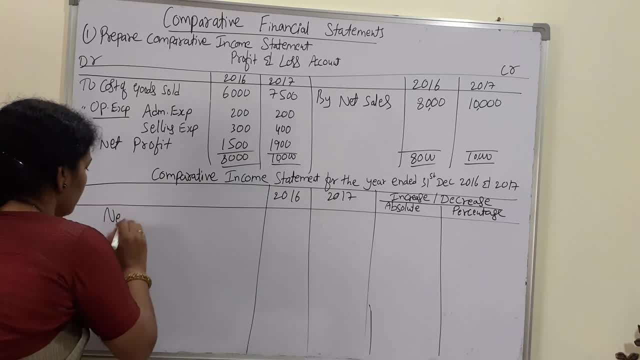 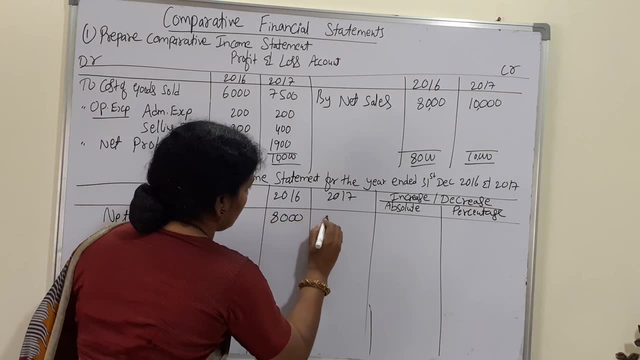 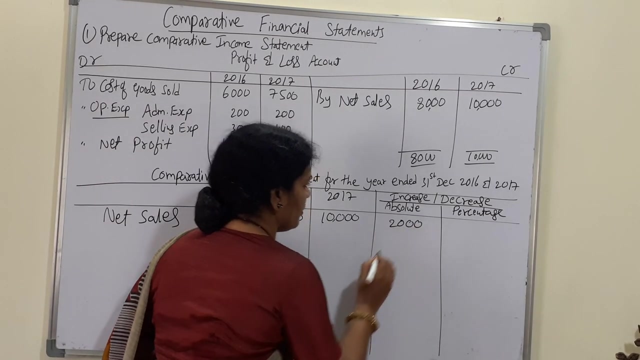 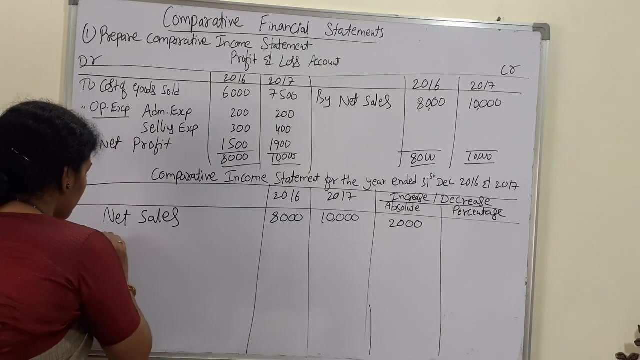 sales will take. net sales are 8,000 and 10,000, so it's increases 2,000. percentage will calculate later. first let us work out the performer: net sales minus cost of goods sold. cost of goods sold at six thousand and seven thousand net sales. 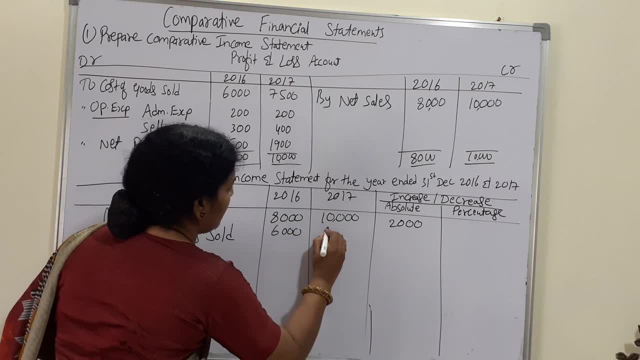 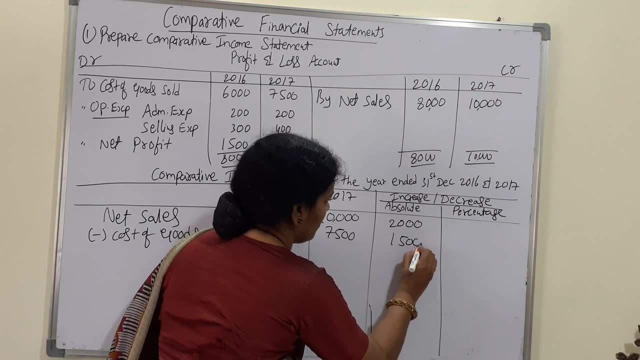 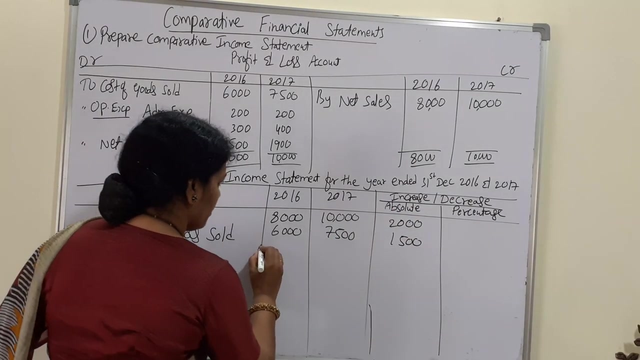 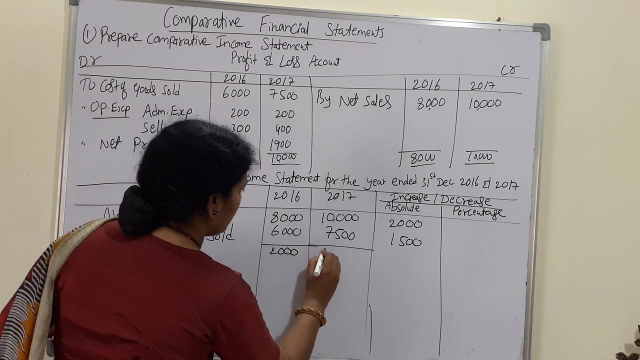 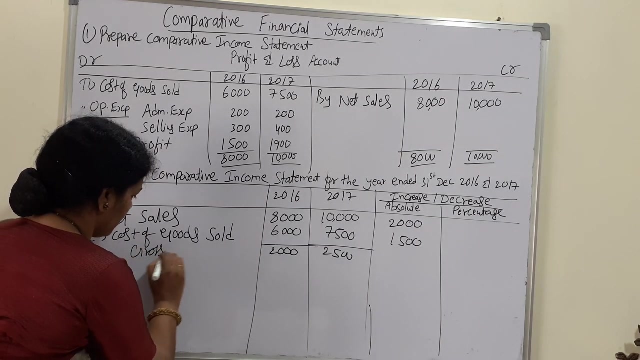 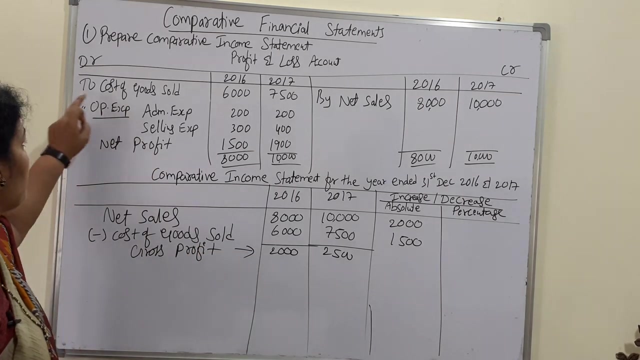 goods sold at 6000 and 7500, so it's 1500. whether increase or decrease will be writing in the absolute and percentage will do later. so now what is this? if we deduct, it will be getting 2000 and here 2500. so this is gross profit. from gross profit will deduct the expenses. 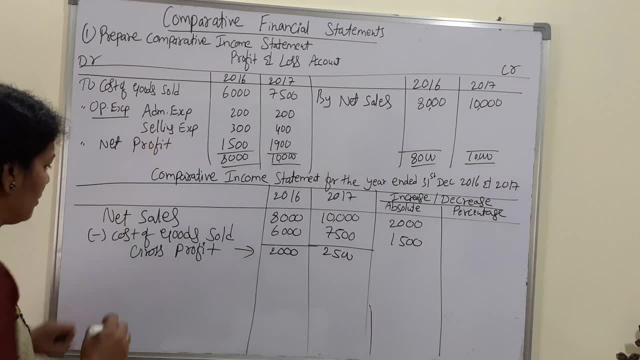 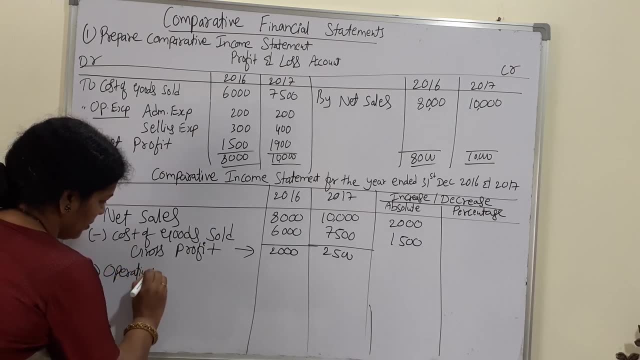 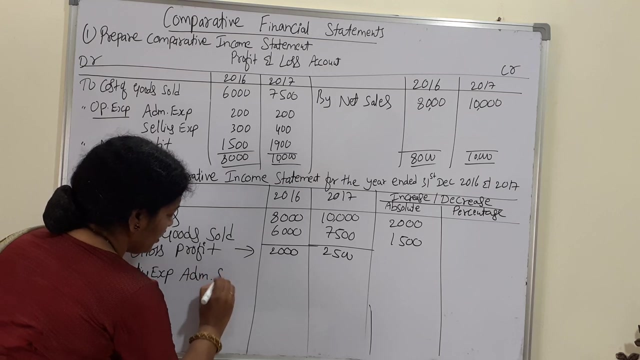 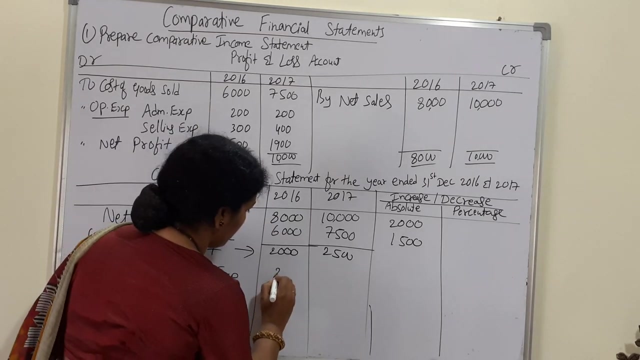 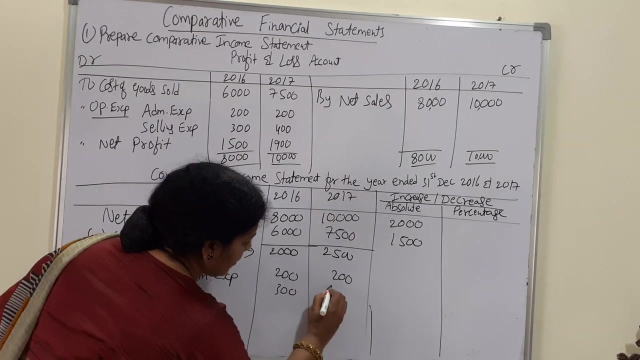 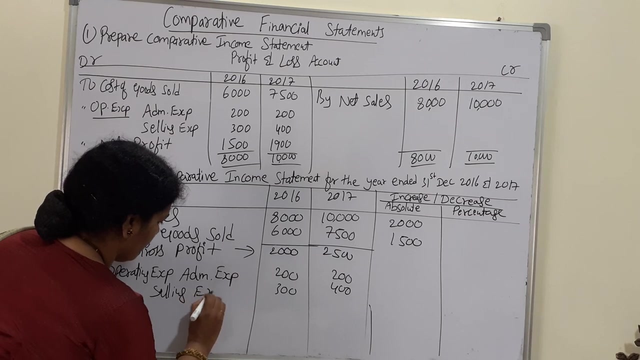 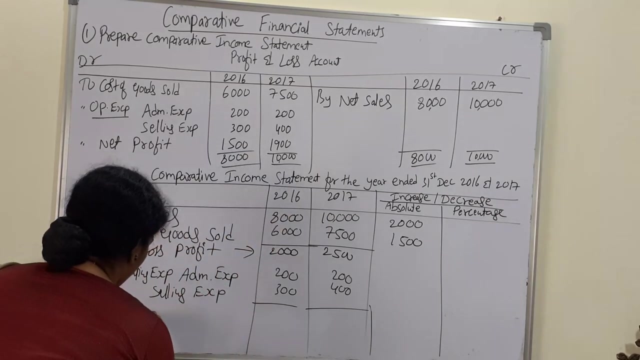 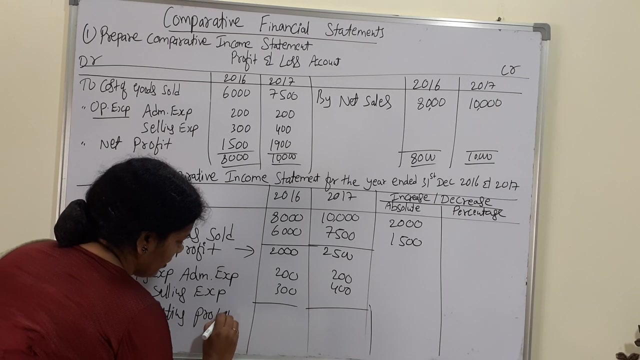 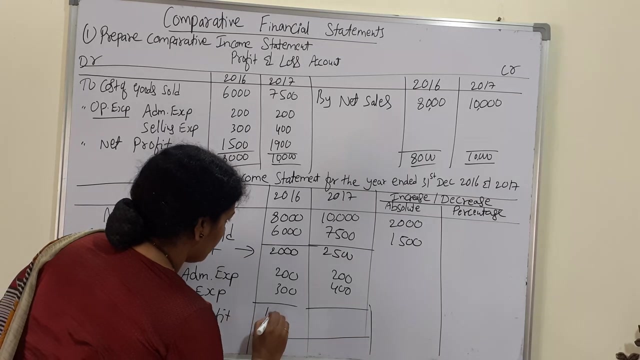 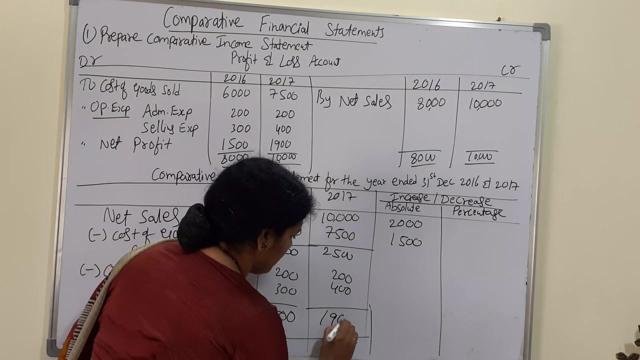 what are the expenses? administrative expenses and selling expenses minus. you can say operating in administrative expenses. administrative expenses 200 and 200. next one is selling expenses 300 and 400. so these two expenses, if you did it will get operating profit. this is operating profit. so 2000 minus 500 will be getting 1500, and here 2000 minus 600 means 1900. so 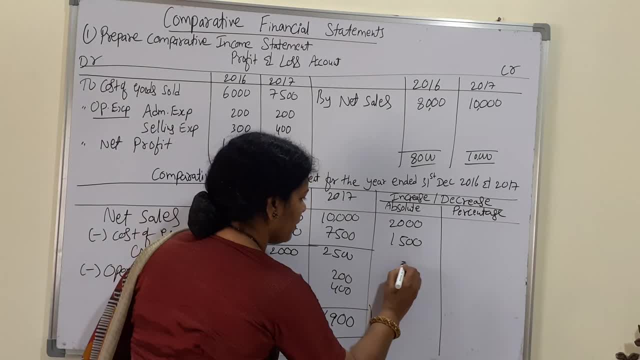 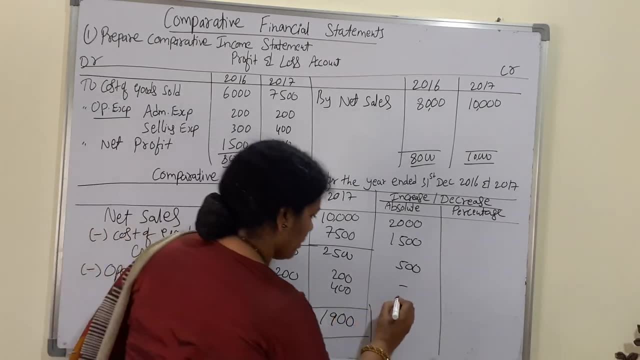 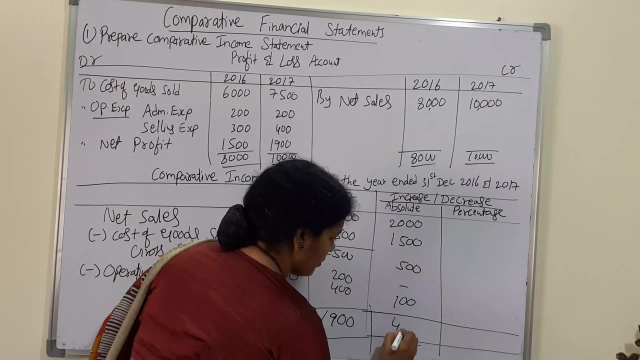 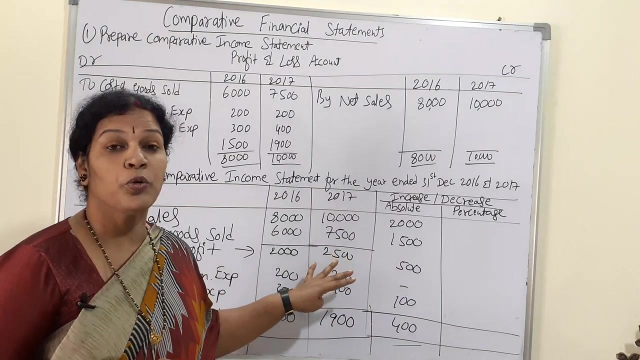 changes. also will write: here gross profit is 500 increased and here no change. 300. 400 means 100 increased and here 400 increased. so this is normal thing we have done. now we have to calculate the percentage, how much it is increased, to get the percentage, always remember how much change is there. 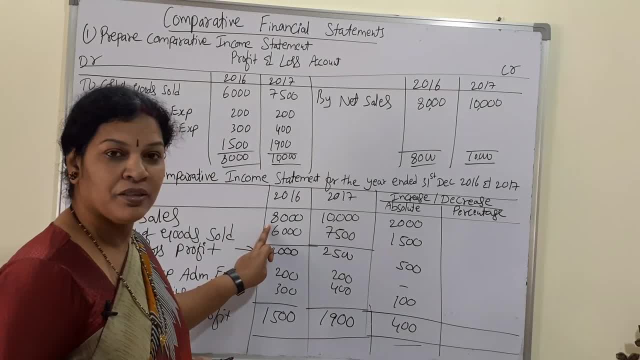 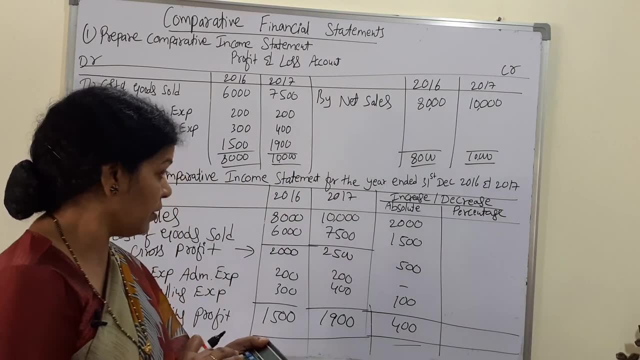 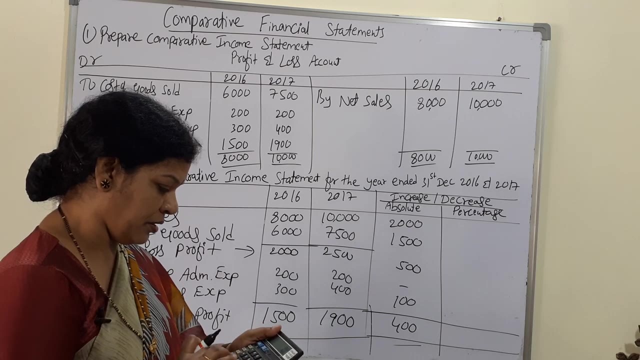 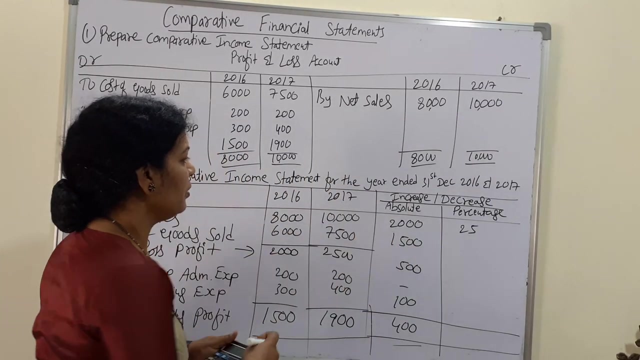 difference, that difference divided by the base 2000 divided by 8000 into 100- we'll use the calculator- 2000 divided by 8000 into 100, it comes to 25 percent. how do you got 25 percent 2000? I'll write it here. otherwise, 2000 divided by: 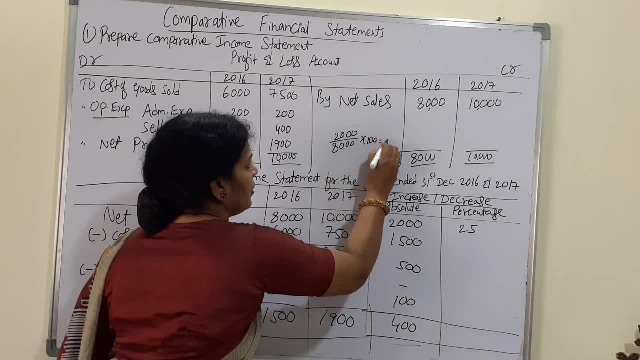 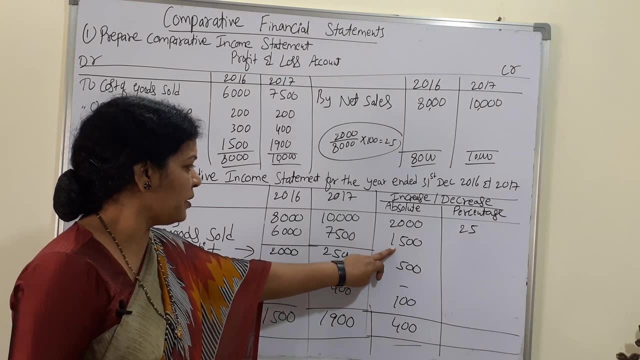 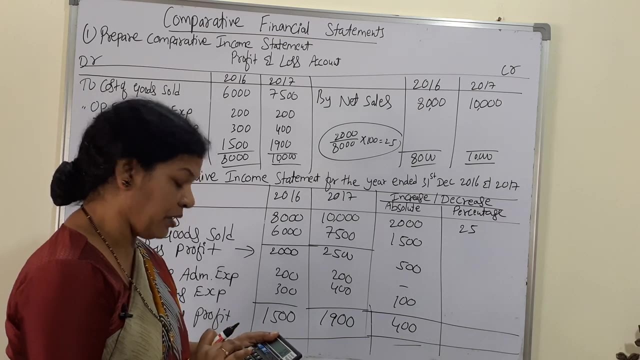 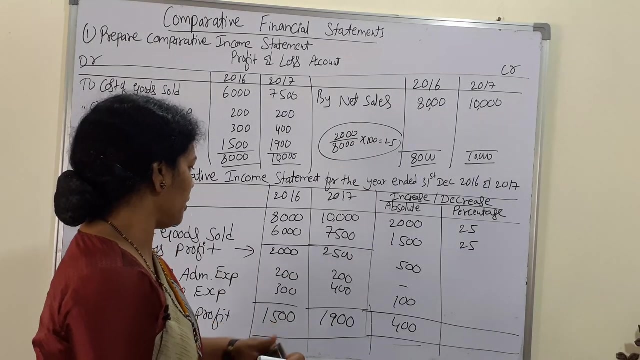 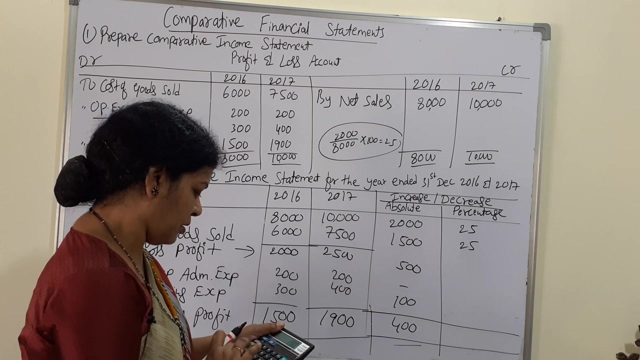 8000 into 100, we got 25 percent. in the same way, every percentage we have to calculate. second one is 1500 divided by 6000. 1500 divided by 6000 into 100, this is also 25 percent. next change: change: that is gross profit: 500 divided by 2000 into 100. this 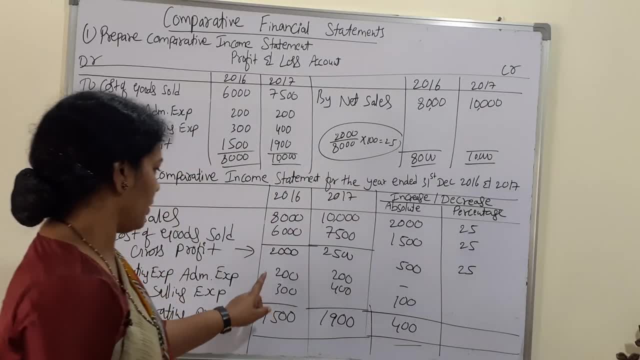 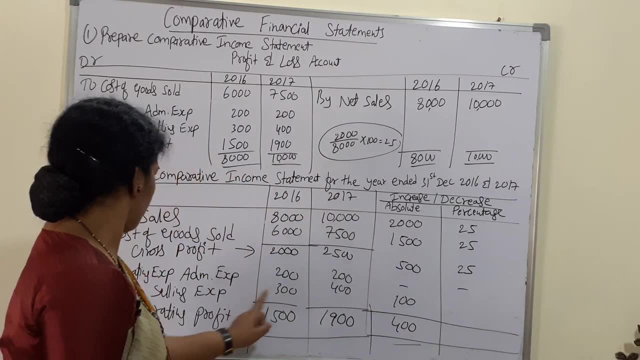 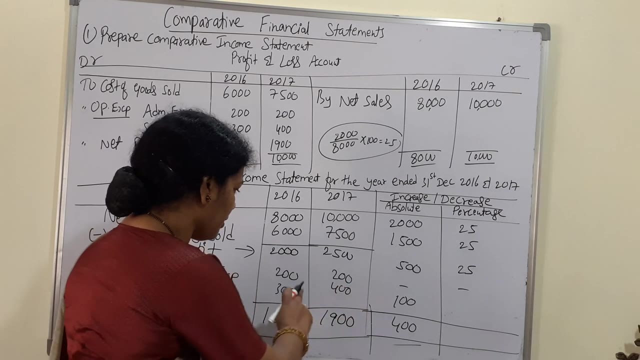 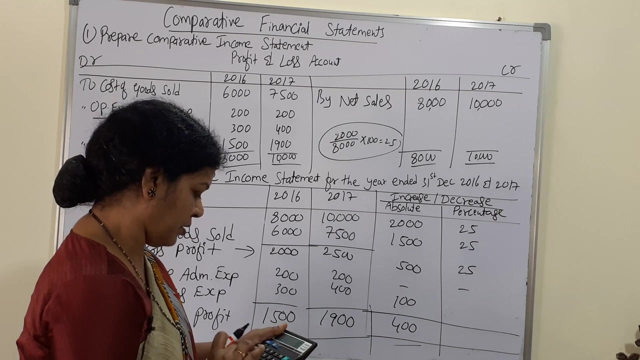 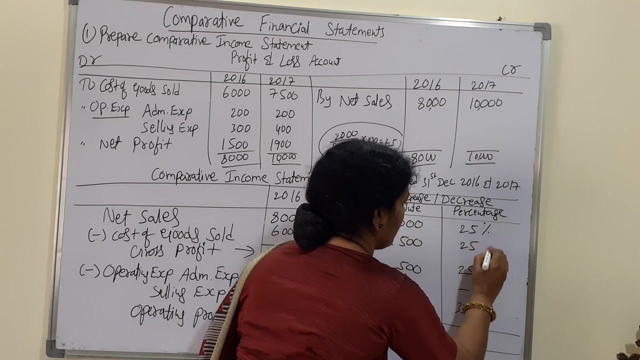 is also 25 percent. then after that change the percentage of gross profit, after that operating expenses, there is no change at all. so it's nearly next one. this is selling expenses. hundred, hundred divided by three, three hundred into hundred, it is 33 percent. that is three point three, three percent. 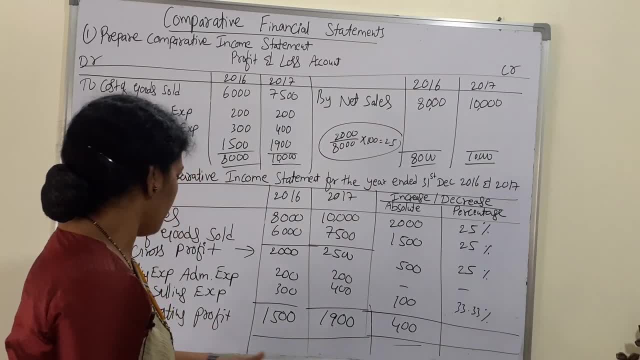 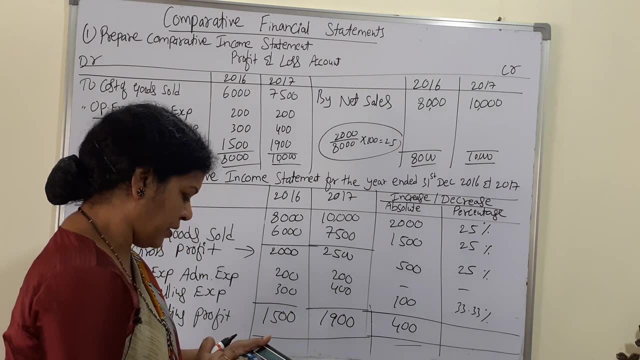 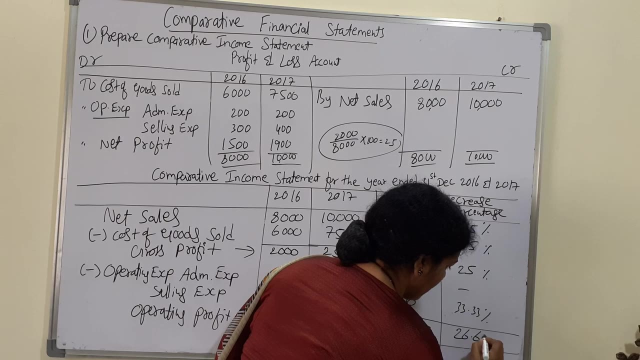 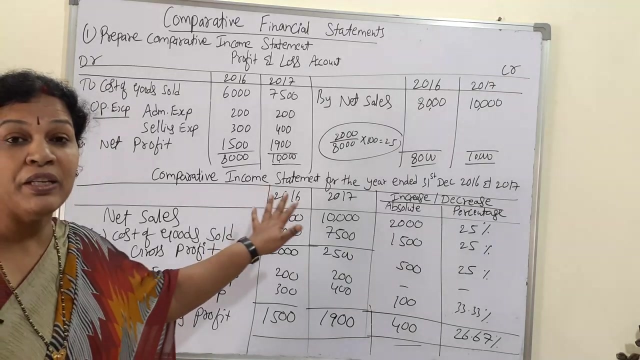 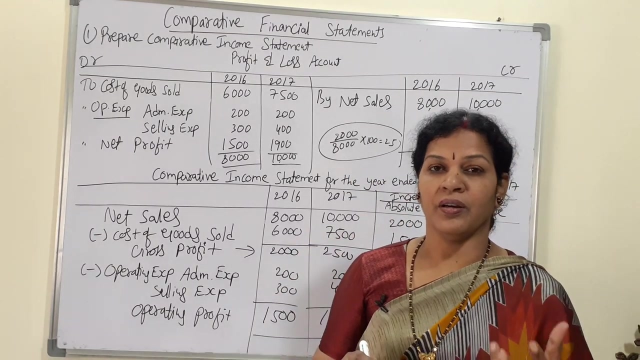 you next. lastly, operating profit 400 divided by 1500 into hundred, this 26.6, means twenty six point six, seven percent. so like we have calculated this of comparative income statement, let me give you a recap then after that I'll tell you how to give the narration or interpretation of the income statement. 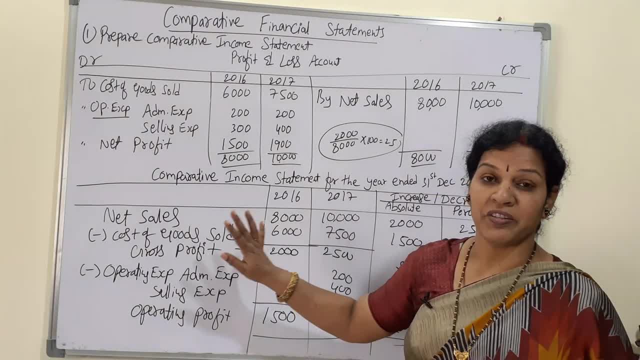 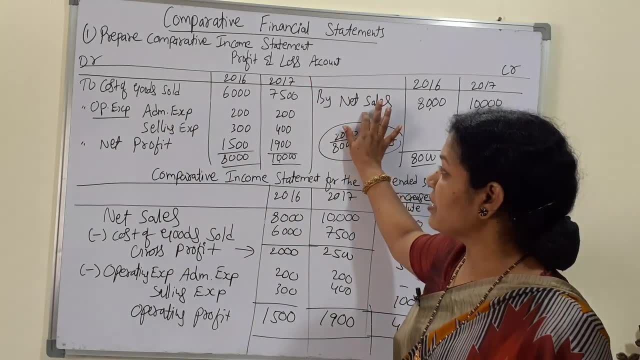 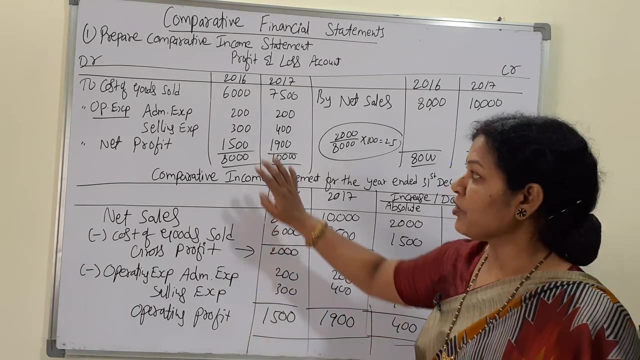 how to give the interpretation. first of all understand what is income statement. income statement will be preparing from the profit and loss account here. from here we have taken first net sales minus cost of goods sold. net sales minus cost of goods sold. we got the gross profit from the gross profit other operating. 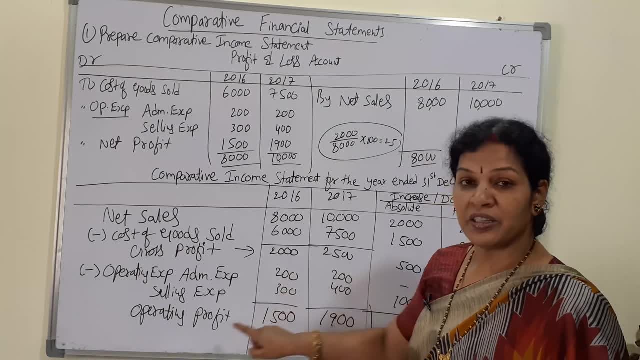 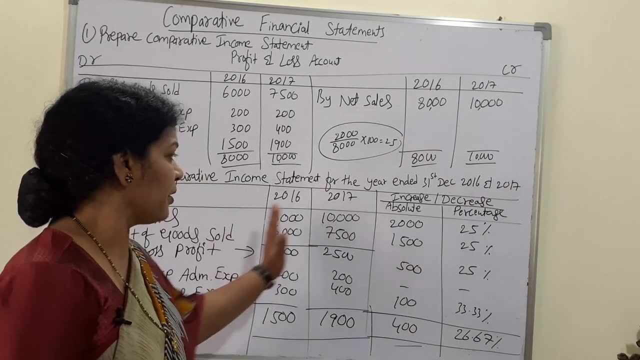 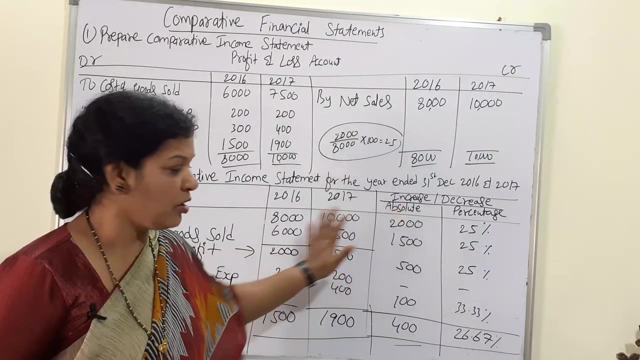 expenses like administrative selling expenses. both we have deducted. we got the operating profit. that's it. so this is the base. now, for two years we have done this, 2016 and 17. now in this another column we are writing absolute increase or decrease, how much is increasing or decreasing? that we have written and this percentage percentage. 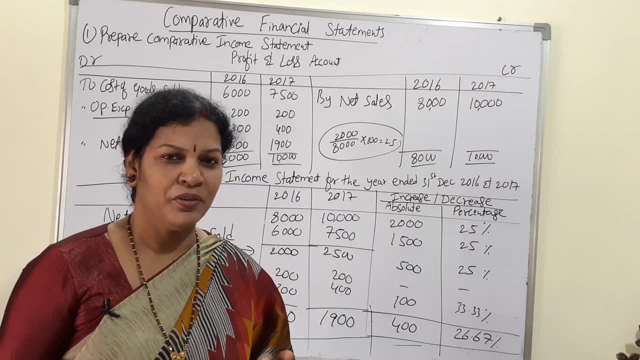 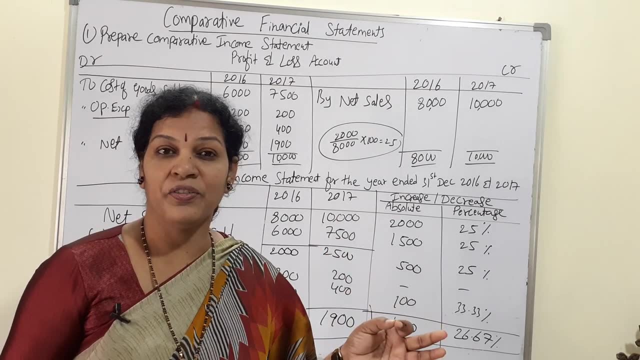 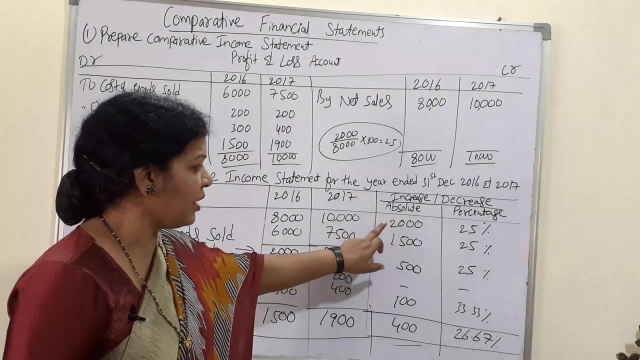 wise generally will understand very easily. if you say calculations, amount, how much is increasing, a normal man cannot understand, even a layman can understand if you say it in percentage wise. so that is why we are preparing percentage. how do we got percentage? the first one is that 2000 means the change increase or decrease that change divided by base. 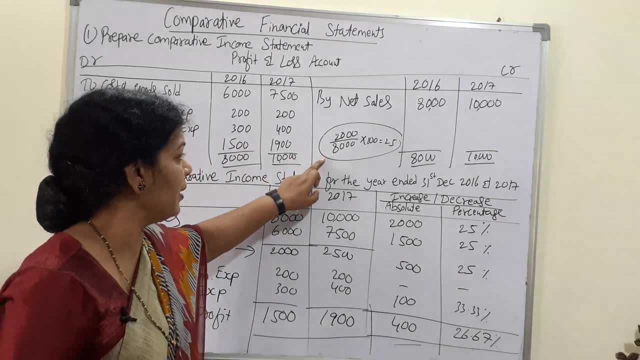 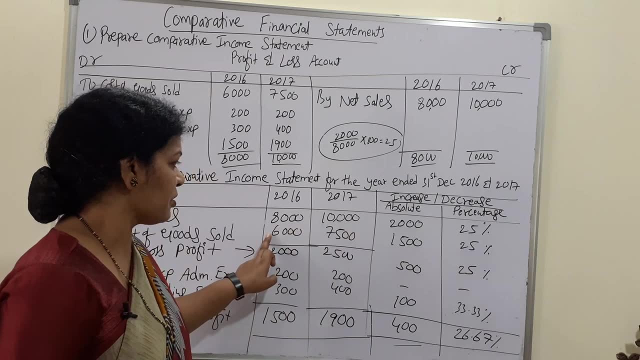 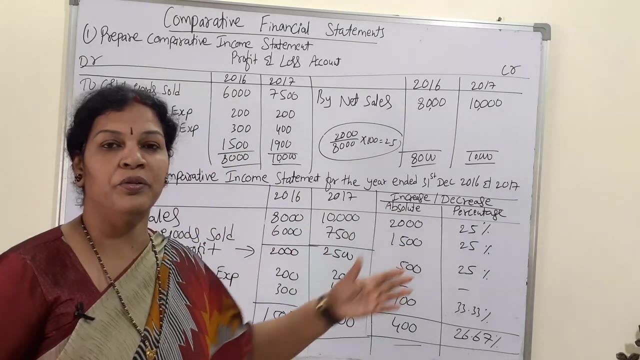 year into 100, as I have done: 2000 by 8000 into 100, 2000 by 8000 into 125 percent. here also 1500 divided by 6000 into 125 percent, like everything this. divided by this into 100, you got the percentage. that's it once, if you prepare. 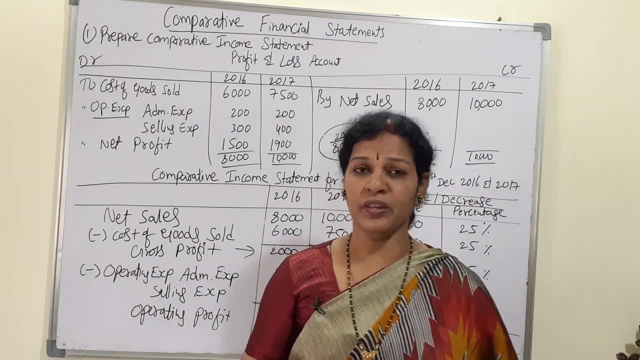 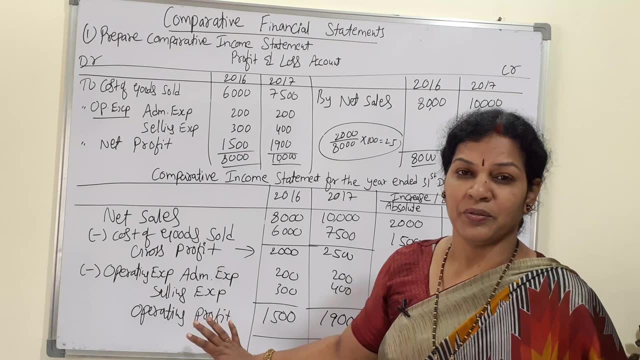 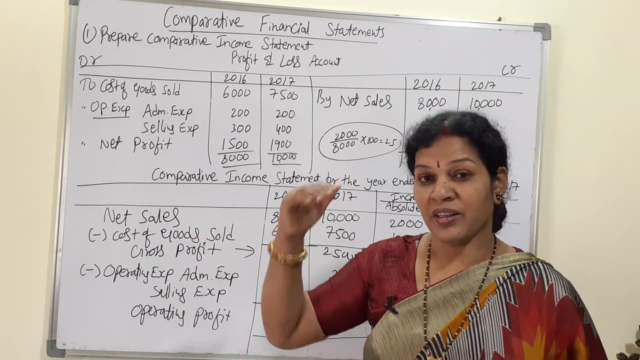 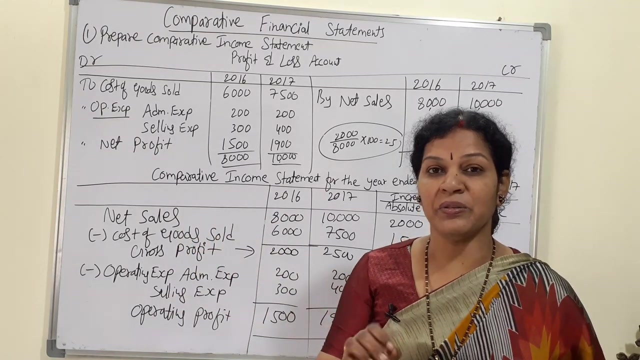 this income statement. you have to give the interpretation. interpretation means nothing but explanation. that what it is, what it is saying, what is the meaning of this? suppose you are an accountant, management accountant prepared this the company managers, CEOs- they cannot understand by looking at this. for that purpose we have to give some interpretation. downside of the problem: 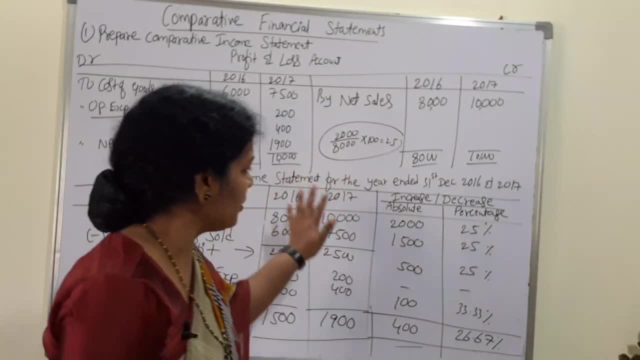 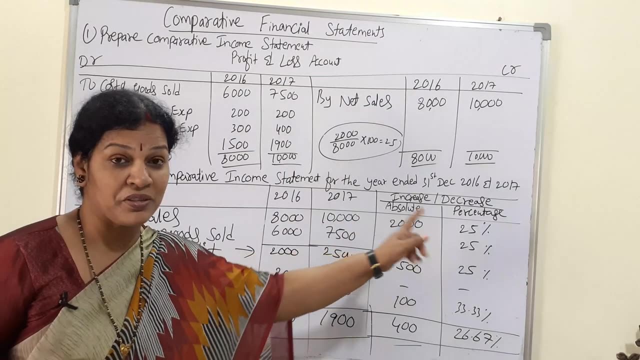 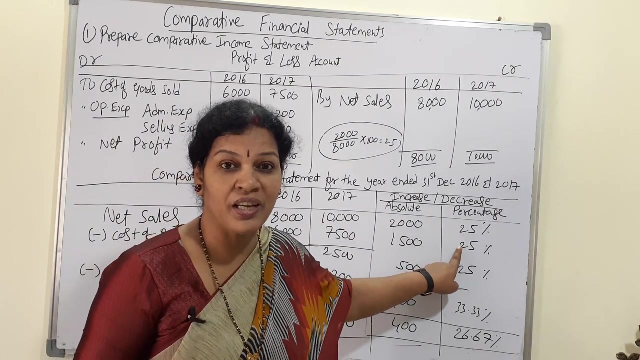 how to give the interpretation. say, you just observe this income statement. income statement is here. first, sales are there. sales are increasing by 25 percent. in one year means 2016 to 17 year. it's increasing 25 percent. it's a good sign. one year in the same way, you can see the 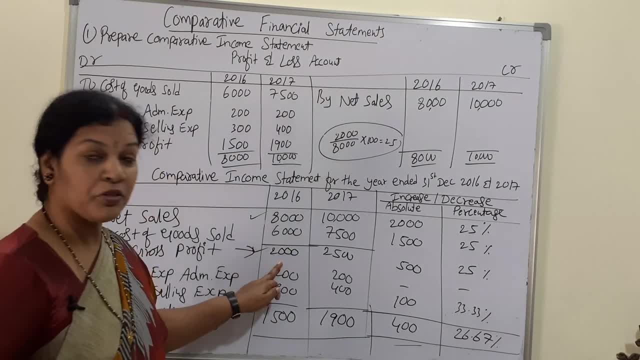 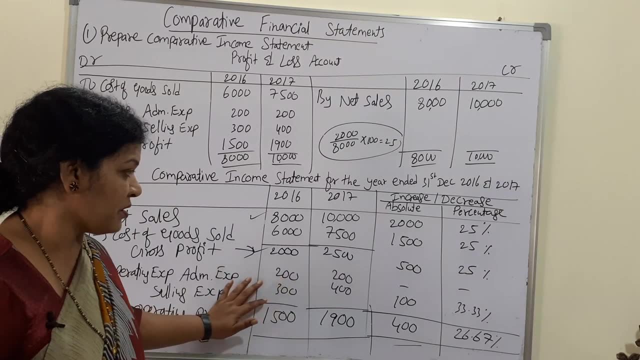 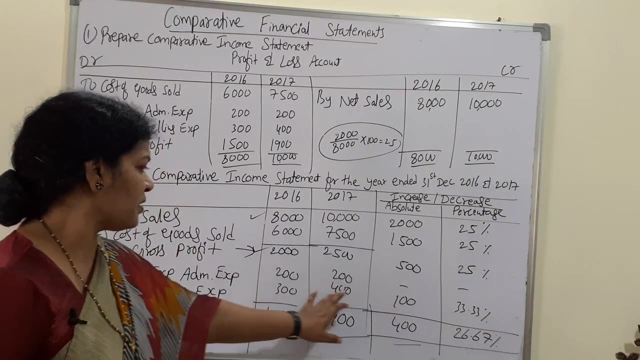 gross profit for sales. we have seen, and GP gross profit. gross profit is also increasing by 25 percent, so it's a good sign. in the same way, operating expenses, expenses, administrative expenses, is no increase at all. as it is next, selling expenses are increased by 33 percent. and lastly, lastly, what you have to give the 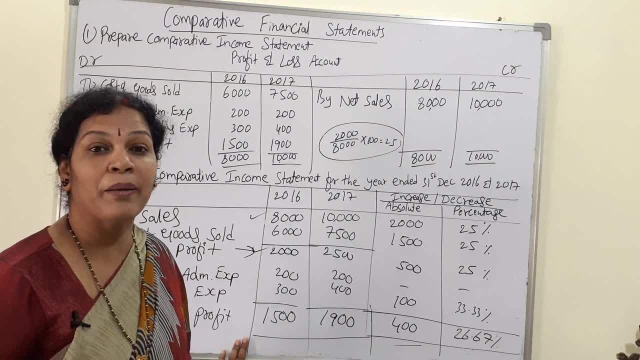 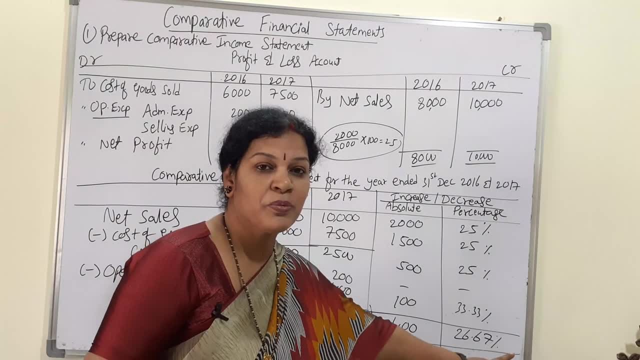 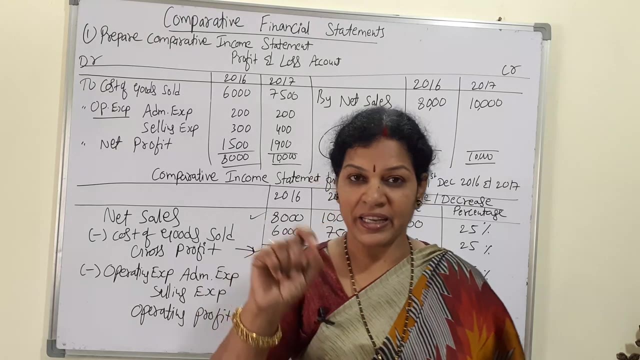 conclusion is that operating profit, which is the main backbone, which main important aspect of any financial company, so that's operating profit, is increasing by 26.67 percent in one year, which is a very good sign for the organization. like you have to give a small paragraph interpretation for this. that's it. this is comparative income statement. 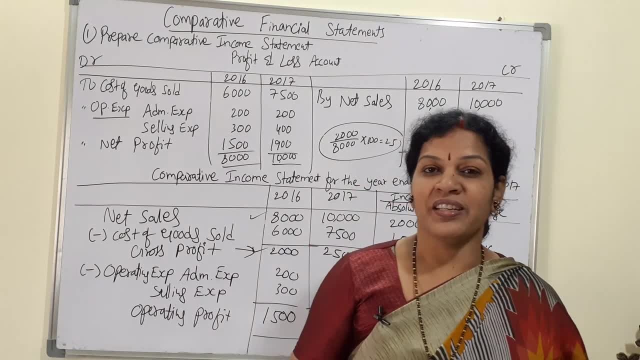 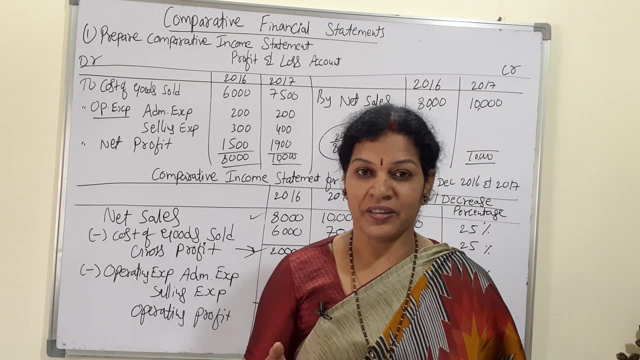 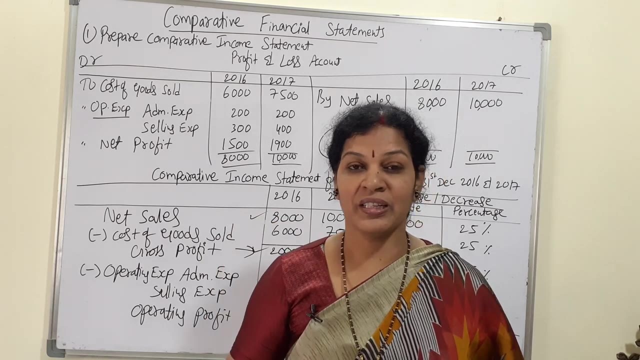 very clear. in the coming class- next class- we'll see comparative balance sheet, then after that we'll go for trend trend analysis and common size statements. also for more subject, more topics: please see the description box or otherwise go to the playlist. you will find serial number weis- a lot of topics, so please do share. 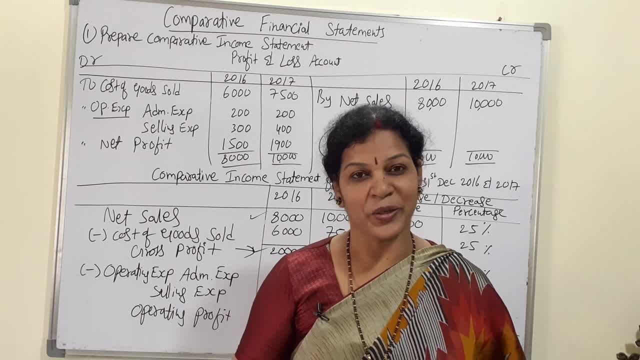 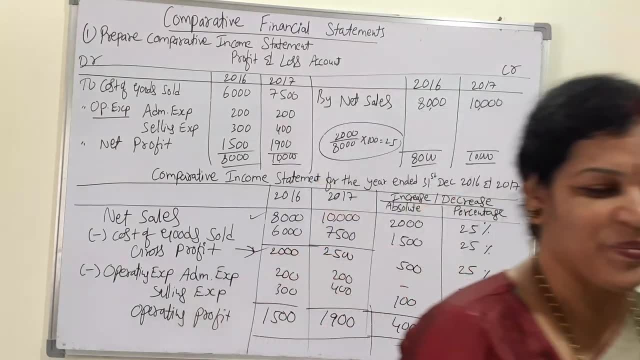 this video with everyone and who are struggling to learn. thank you very much for your feedback. stay in touch with me for more subjects. wish you good luck, practice well.